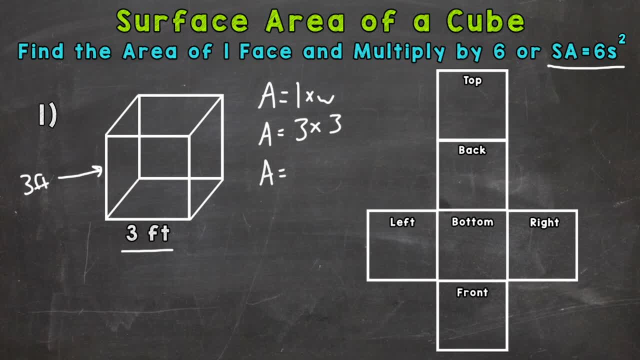 So we can do three times three to find the area of one face, And three times three is nine. So the area of- let's say we did the front face there, the area of that front face is nine square feet. So over here to the right I laid out a net of that. 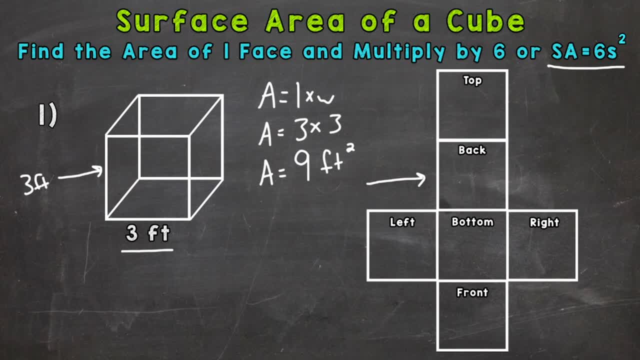 cube. A net is when you unfold a 3D figure, so we can kind of better visualize what we're doing here. So the front has an area of nine square feet. So we need to find the area of one face, to find the surface area, again, the area of all the faces, so we can think of it. 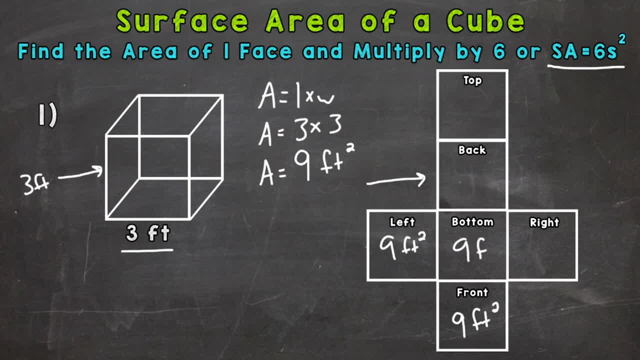 as all the faces having an area of 9 square feet. so if you kind of picture folding that net up, we would just get this cube right here. so 9 times 6 is going to give us the surface area. so we could do. surface area equals 9 times 6 and 9 times 6 gives us an answer of 54. 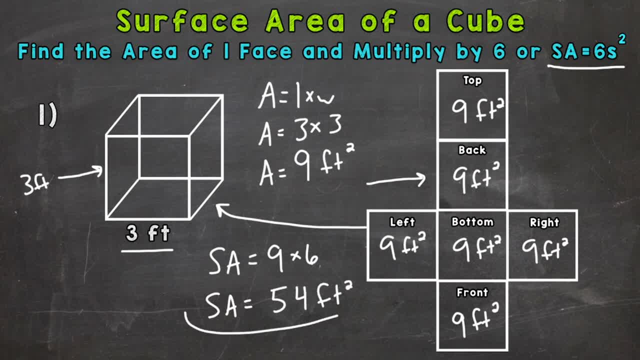 square feet. so again we found the area of one face, the front here, and we have 6 faces total. so we multiply that 9 by 6 to give us the total surface area. now i'm going to show you how to use the formula too we can do. surface area equals 6 times a side length squared. so 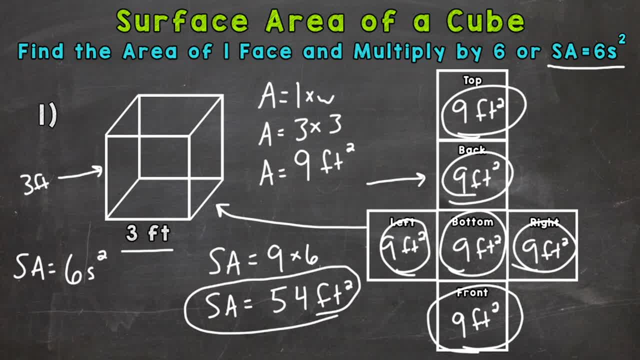 that s squared, or 3 squared in this case, gives us the area of one of the faces. it's the same as doing length times width for a square. so we can plug in one of our side lengths, which is 3 feet, So 6 times 3 squared. Now, due to order of operations, we need to do 3 squared first. 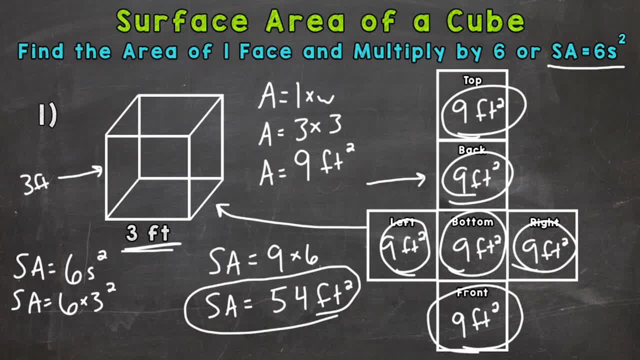 which is 3 times 3 is 9, and then multiply by 6.. So we get the same answer of 54 square feet if we use the formula as well. So there you have it. There's how you find the surface area of a.